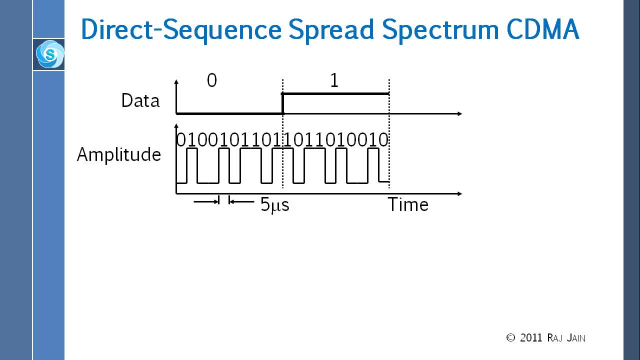 language. You know, if we all spoke English, there will be a lot of noise and we won't be able to understand anybody. But one person spoke English, one person spoke Chinese, one pair spoke Chinese, one Spanish, one Hindi and one Suvannama Sa. There is no interference, right? But everybody. 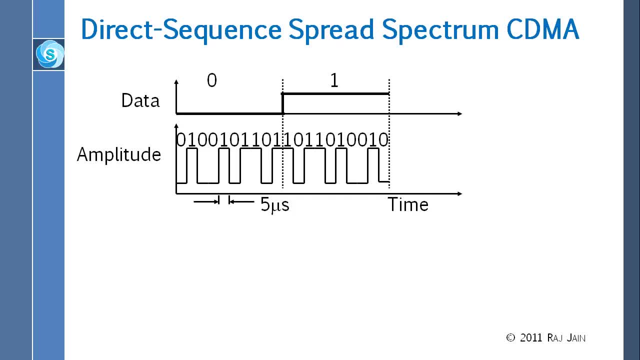 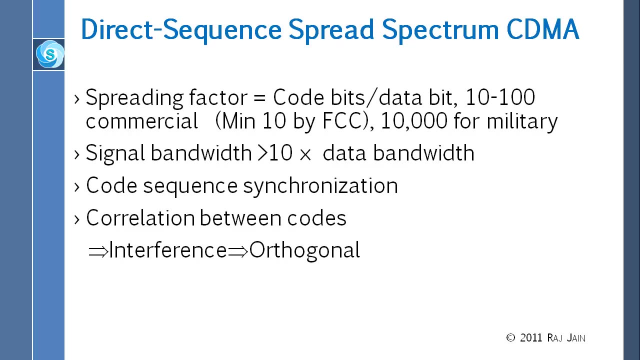 is tuned to their code Right, Everything else doesn't make sense. So when we use a language that is our code- division of multiple access seems like you got this word up there- you have to write for the PC to understand the meaning of theafar. 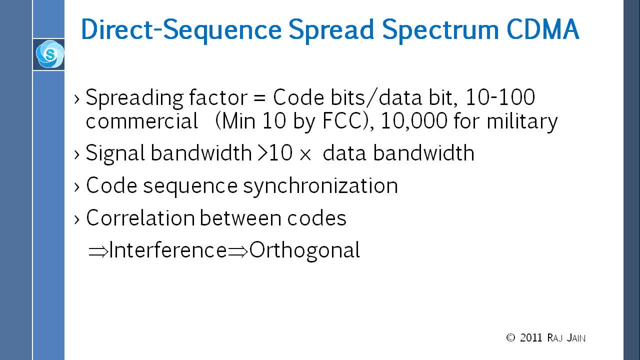 CDMA. So how many bits do you need? Well, 10 bits will let 100,000, will let 2-10,, maybe 1,000 people talk, but that will be too many. So generally we need the codes such that they are: 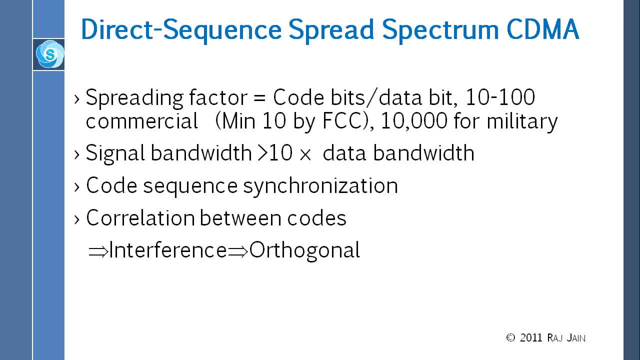 least interfering. I mean, if suppose one spoke Mandarin and one spoke some other version of Chinese, I don't know- then they will interfere. So you really want the codes to be very, very far away? Right, Yeah, then we can all speak. 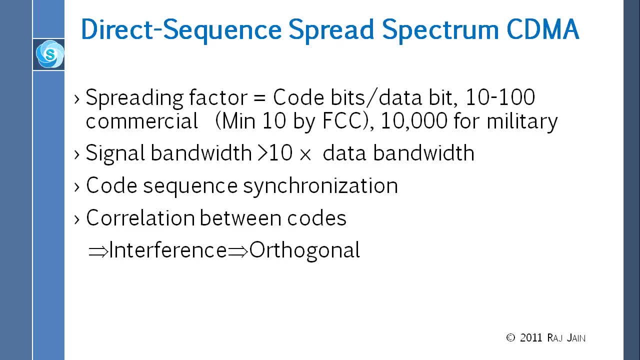 at the same time on the same frequency. That's the point. We don't need to change the frequency. We can all speak at the same time on the same frequency and not interfere. And the more longer code we use, more people can use it at the same time. Yeah, 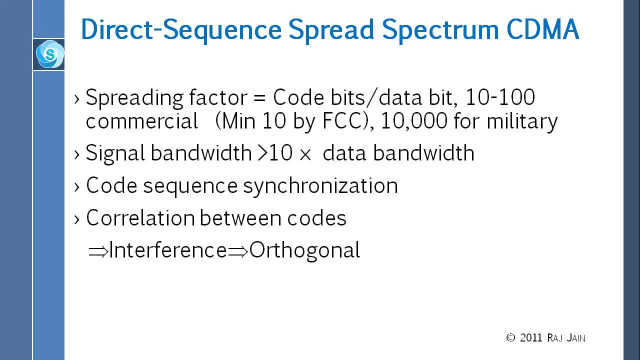 Yeah right, So basically you negotiate that You are allocated. It's like a frequency. How do you know which frequency to use? Somebody tells you that, okay, go ahead, Two of you, please use this frequency. You know, somehow you negotiate that okay. 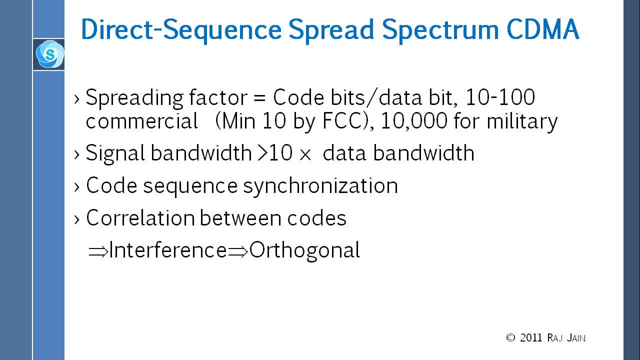 we are going to use this frequency or this code. So once, just like frequency division multiplexing or time division multiplexing, here we have code division multiplexing, And this is the thing. CDMA is the thing that was invented by Qualcomm and that's how they made their billions. 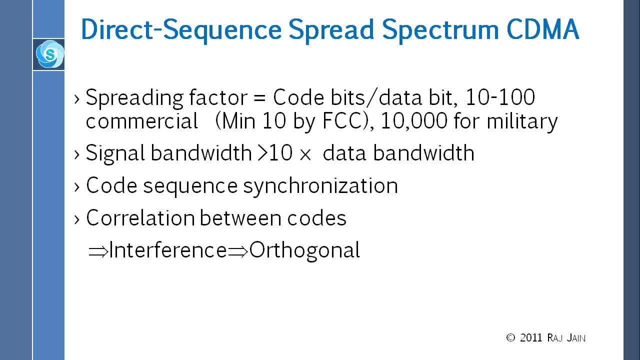 Right, And today, every cell phone, everything that is 3G, uses CDMA. Everything that is 3G uses CDMA. So all of you use 3G, all of you use CDMA, All right. And it is not used in 4G, by the way. 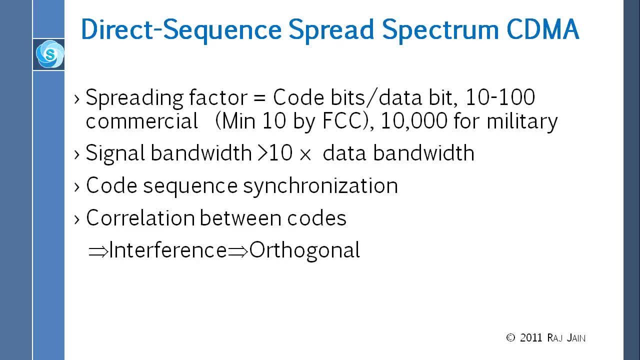 It is not used in 2G, but in 3G, everything is CDMA. What about GSM? GSM is 2G, 2G. Okay, So it turns out in the days of 2G everybody had a different method, but Qualcomm came about right in the 90s. 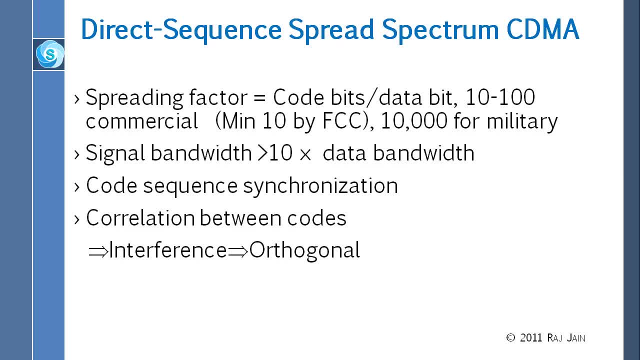 when the 2G was done and so everybody agreed to 3G. That was the newest technology, 95 or something like that some year. So 3G all over the world is CDMA And 4G again gave up on CDMA. 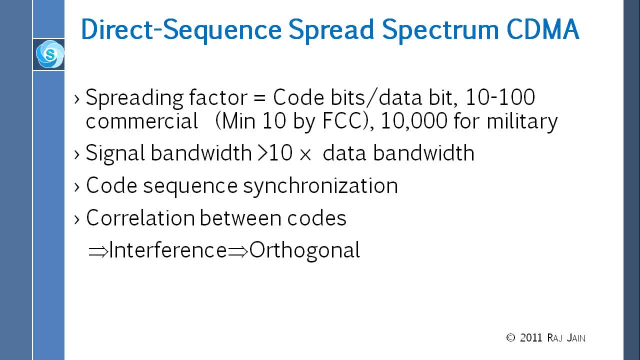 and they adopted something else which we will not teach In this course. I'm not going to even spell that word, But that one 4G got rid of whole CDMA thing. But for 3G we have CDMA. 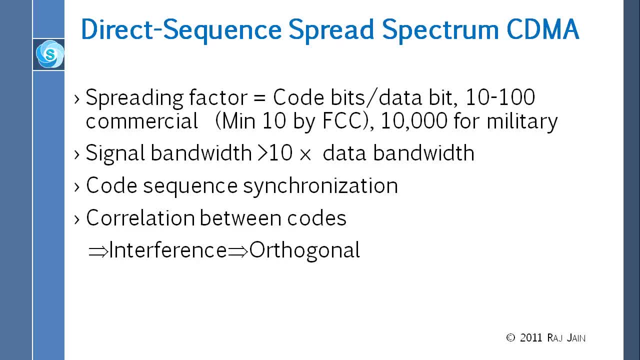 So signal bandwidth. now, here is the problem with this, though. Now you are sending bits which are very, very small. if you want to call these bits, We don't call them bits, We call them chips. You break a bit into chips. 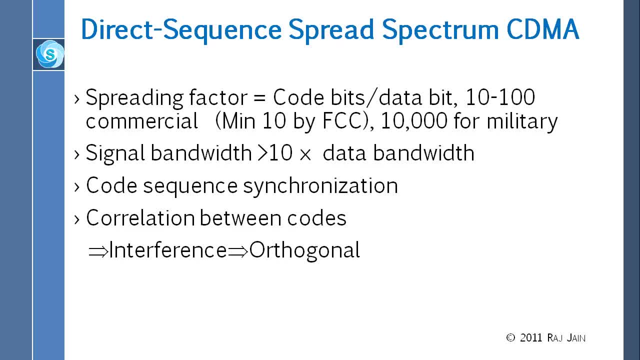 So there are 10 chips per bit here, as shown, And military will use 10,000 bits because they really don't want anybody to know their code. So they use lots of chips. We use 10 chips And we need to basically synchronize like he asked. 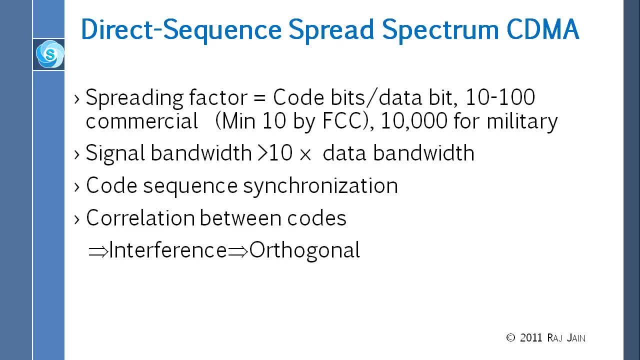 that you know. how do we know? So we need to have some negotiation beforehand to select the code, And we want to make sure that the codes are not selected very close to somebody else, Otherwise we'll be interfering. So we need the codes which are orthogonal. 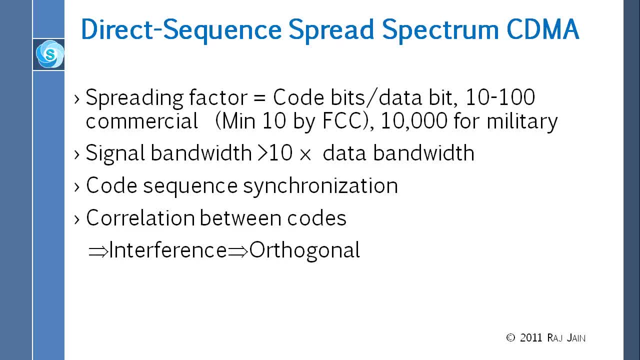 Orthogonal means they don't affect at all perpendicular. Now what that means is that if you take 10 bits, you'll find only a certain number of codes which don't interfere with each other, And again, we are not going to go into that detail as to what that means. 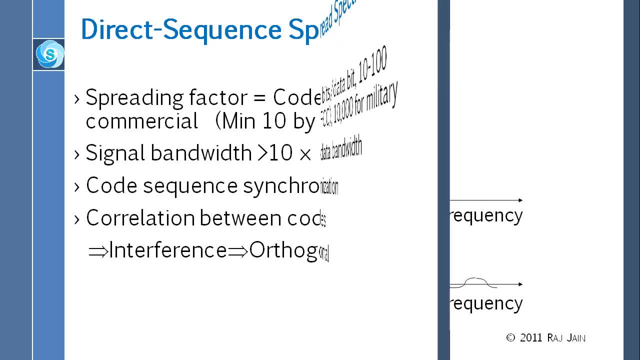 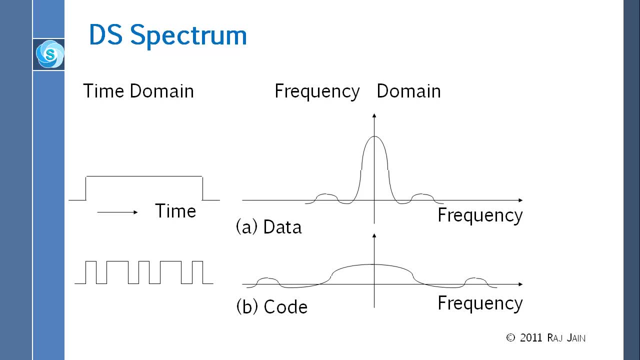 because there is a lot of coding theory in there. But one thing you can understand very easily is that if you are not doing, if you are not doing, the CDMA, then your bits will be long. And if you were to look into the frequency domain, 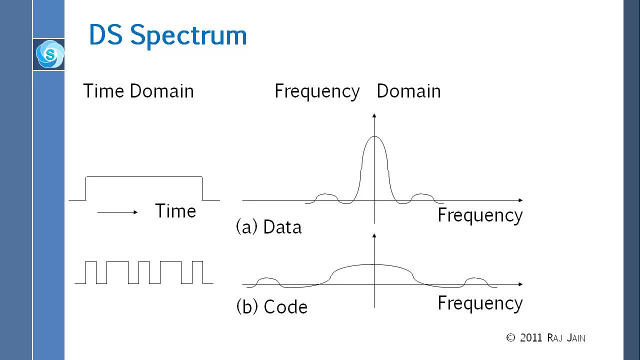 then the frequency domain spectrum will look like this: where you have lot of energy, lot of power at certain frequency, This is basically: if suppose you do 10 bits per second, then basically at 10 hertz you will see lot of power. 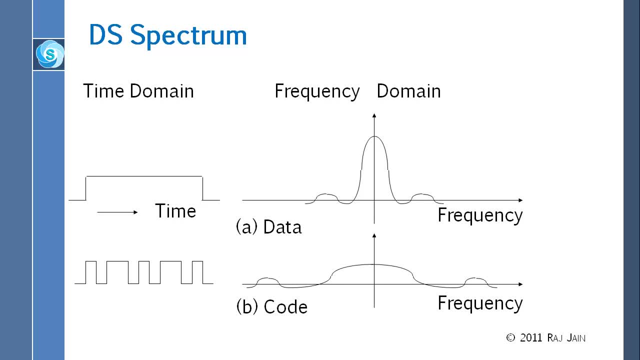 On the other hand, if you do this, which is instead of 1 bit, you send 10 bits. now you have power spread all over. It's not just here. there is high power, but it is much wider. This is much narrower. 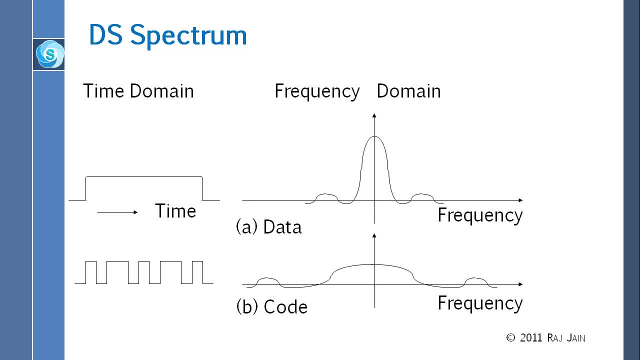 Right, So that is why it is also called spread spectrum. We have spreaded the spectrum, We have spreaded over the spectrum. Everybody is using the same spectrum and they are, so they are spread and they are using different codes. Okay, 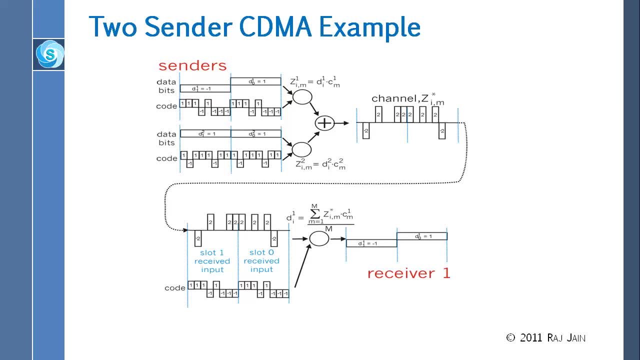 So here is an example from the book. So this sender selects this code and it sends minus 1 and plus 1.. Minus 1 and plus 1.. And it is better to say minus 1 plus 1, because then you can easily add, multiply two different codes. 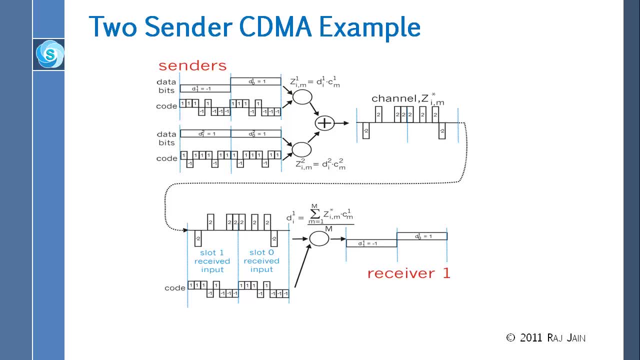 So this is one user, This is second user. This is different code, This is a different code. So this user, So this user- has minus 1, that code plus 1, just the opposite code. This user has minus 1, this code plus 1, the opposite code. 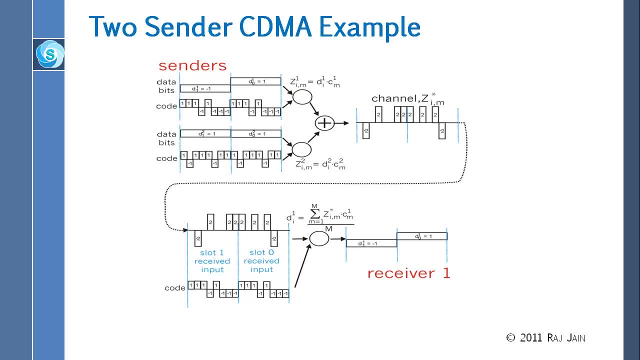 When they are both transmitting on the wire, things mix up and instead of 1, minus 1,, 1, minus 1, you get 2, minus 2, plus 2, something like that, because you add up. 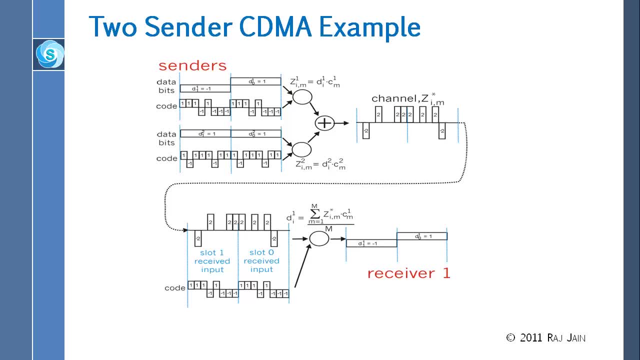 So in the first slot, in the first chip, this one sends minus and its code is 1, so it gives you minus 1 there. and this one sends minus also, and its code is 1, so it also sends minus 1,. 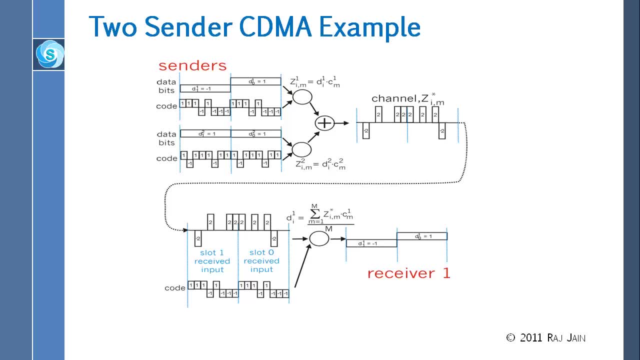 so this one sends minus 2.. And so on and so forth. So you can basically write down that this is what is on the wire, It is on the air, It goes all the way here and now. each of these people correlate with this code. 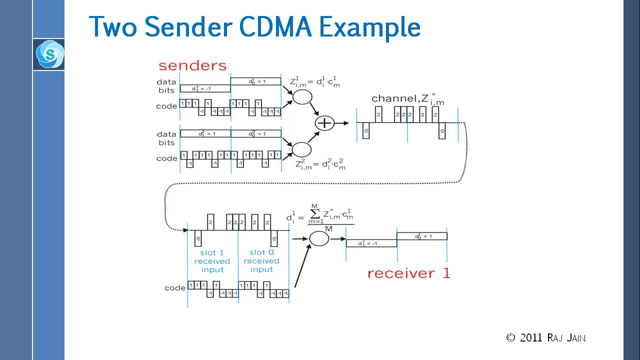 So this person, whichever this person is, 3 ones, is this first person. First person multiplies correlates with this code and after the correlation it figures out that minus 1 was sent. Okay, In the first slot and then similarly you can do in the second slot. 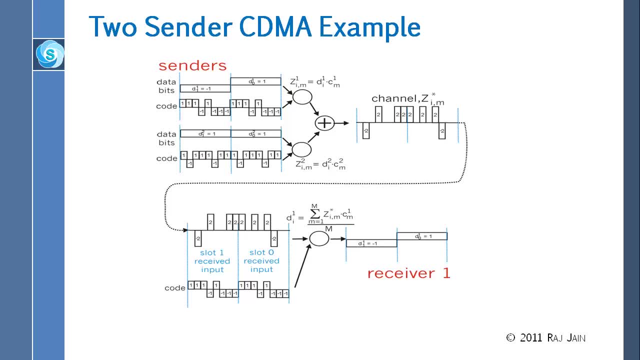 and plus 1 was sent. Yeah, yeah, right, but here the combination. here let me just see: first chip is minus 1, and this one is plus 1, so it is 0.. Okay, The second chip is 1,. 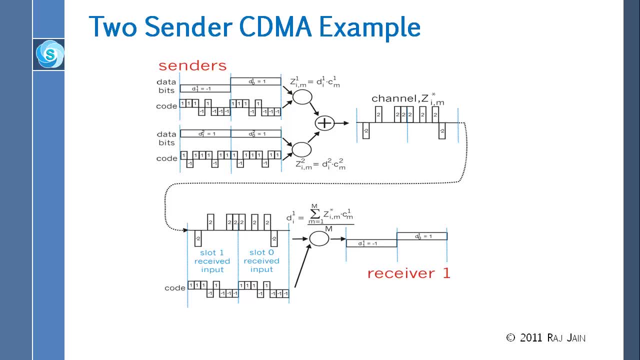 minus 1, and this is minus 1,, so second chip is minus 2.. Okay, So basically what is going to happen is, using that formula, you can calculate what is on the wire, and using similar formula, you can calculate what your person sent. 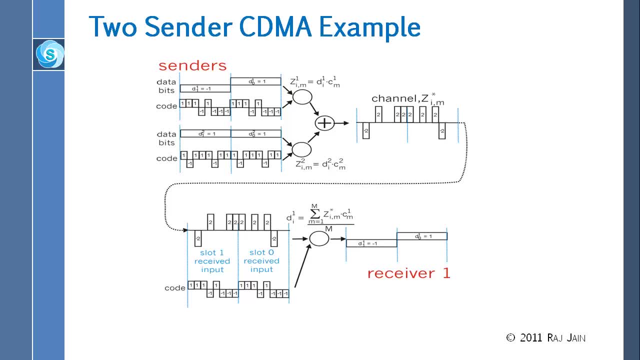 You see, I mean on the air it is minus 2, plus 2, plus 2,, whatever it is right. But this is your code, so you correlate with that and then you get this. You take the code. 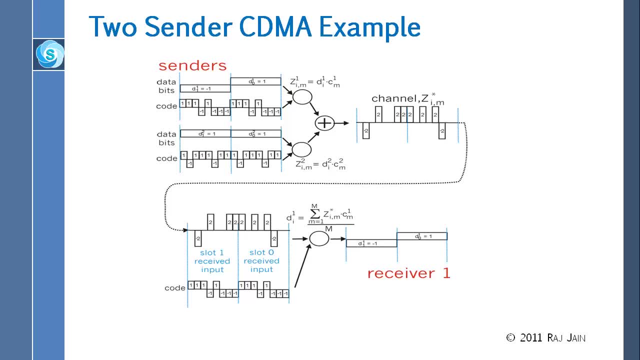 the code is C. Z is on the wire. you do this, for m is equal to 1 through capital M, which is your 10 bits here, and that gives you D And, by the way, it will not give you perfect D. 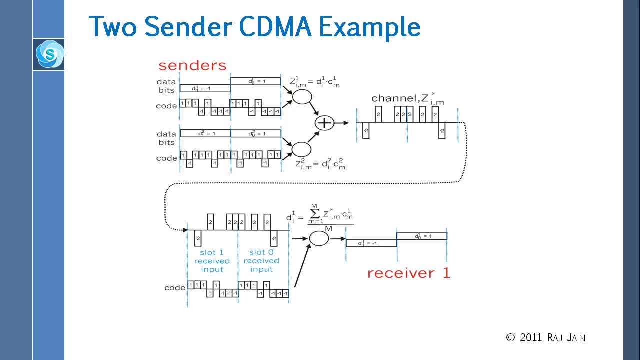 so you will not get 10 minus 1s here. You might get 8 minus 1s and 2 plus 1s, and then you say: okay, this looks like you know minus 1 to me. 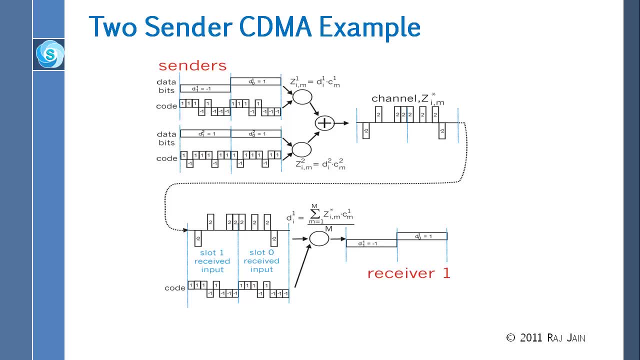 Because of the noise and interferences things are not always perfect as shown in this example. You know you might get few here and there. Yeah, In CPMA everybody broadcasts to everybody and then the receiver, like Not everybody backups everybody. 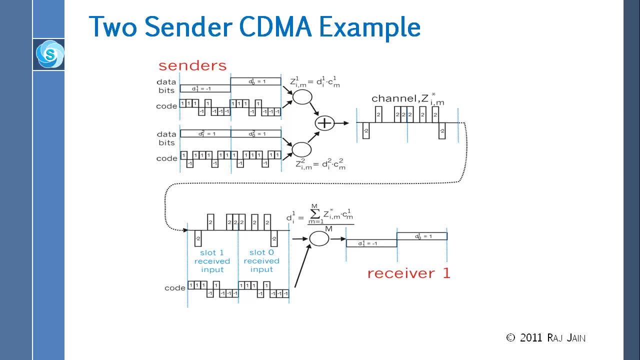 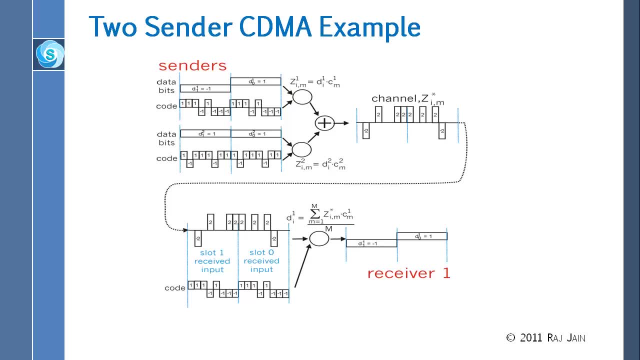 No, the other receiver. you can put another receiver here too, which is not shown, and you can just do the same formula with their code and they will get plus 1, plus 1s. Oh, the receiver decides who he wants to listen. 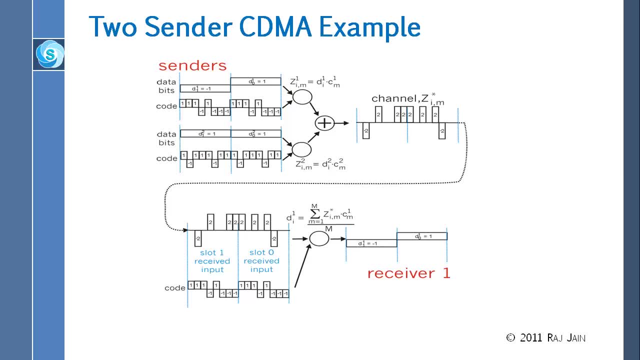 Yeah, well, they are paired right. I mean, the receiver and the sender are the pair and they have decided a code. In fact, it doesn't have to be paired, I mean, if you have two lectures going on in the same classroom. 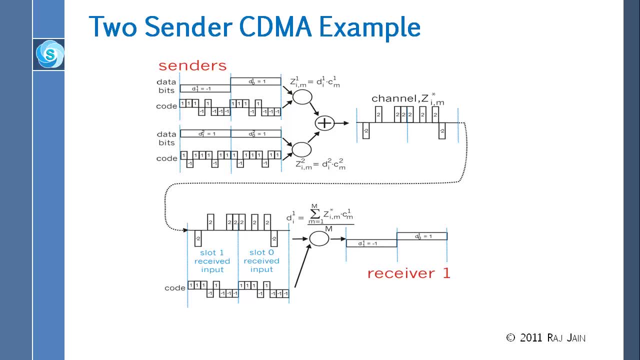 and 60 people want to listen to this lecture and 60 people want to listen to some other lecture. they could use CDMA Again, think you know one lecture could be in Chinese and one could be in English, As long as you correctly do the code. 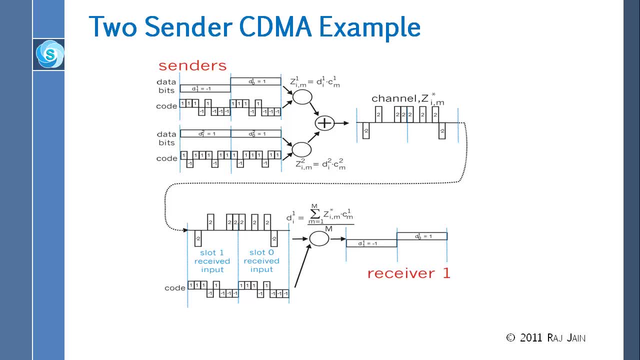 people are not confused. Plus 1, zero, Yeah. so what it did was. the formula says that they tell you add up everything, and when you add up, um, then yeah, you will get minus 1.. Second is: 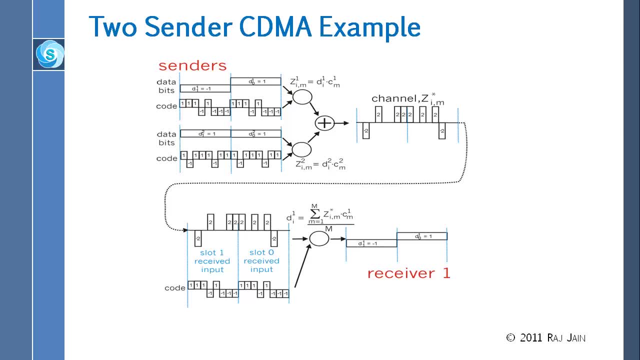 in second half this one, you will get second slot. you will get slot 0 and slot 1.. Let's see the numbers are kind of opposite of: yeah, slot 0 is first. yeah, Slot 0, you will get. 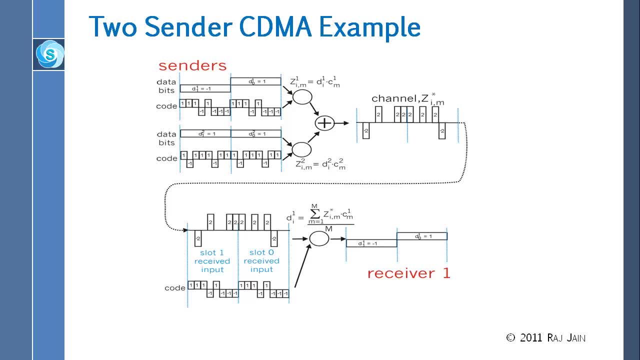 um, whatever you send actually minus and slot 1 would be that one. So this is kind of reverse here. This is slot 1.. This is slot 0.. The CDMA you will get. you will get. 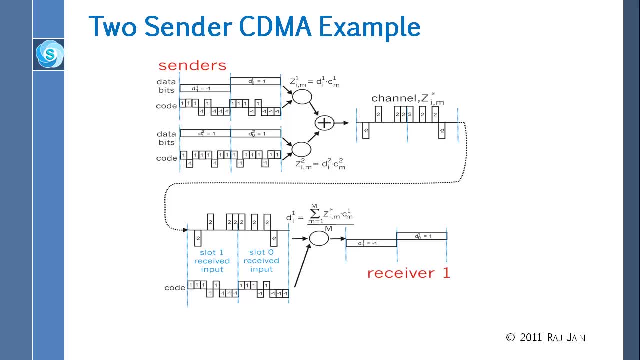 you will get. does CDMA use parity to bit error correction and all that? No, actually, here is the thing: The codes are actually much more protected than parity. So the codes, if you use all 10 bits and you use 1000 users. 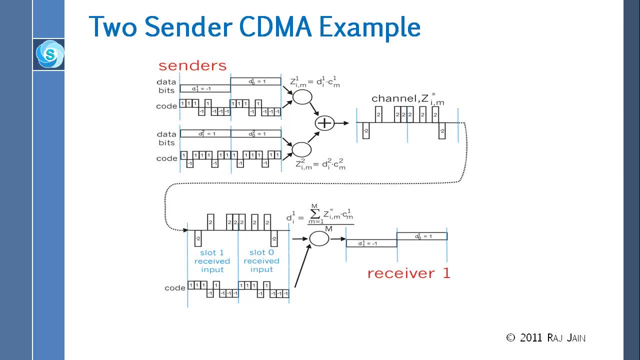 there is no protection. But suppose there, there you use 10 bit code, only 2 users. I mean you are sending 8 redundant bits, So there is lot of redundancy. So it will correct lots of errors. 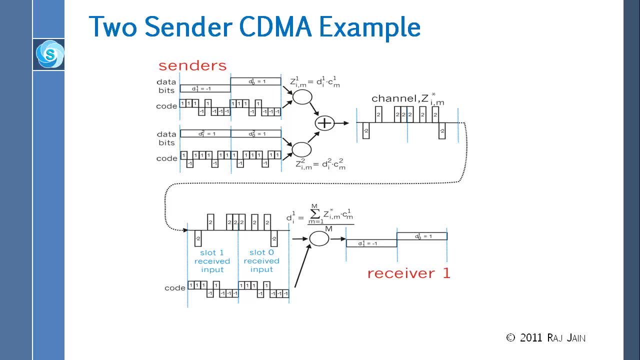 Well, and you don't correct it. but basically what? as I said before, the numbers will not come out perfect, But there will be if any time is more than 5, you say it is 10. You know.